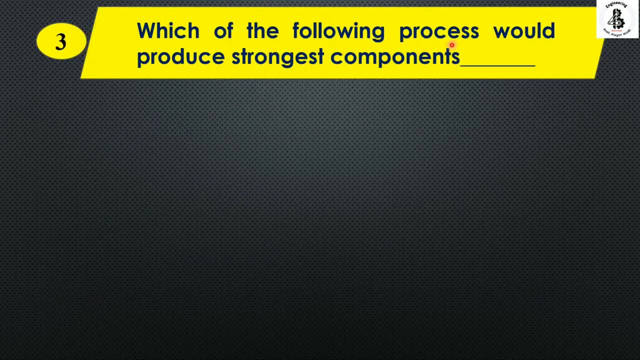 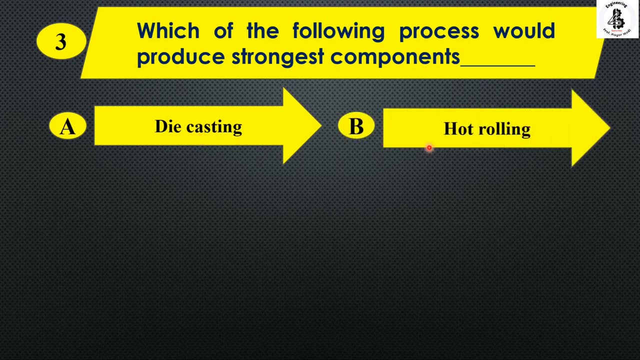 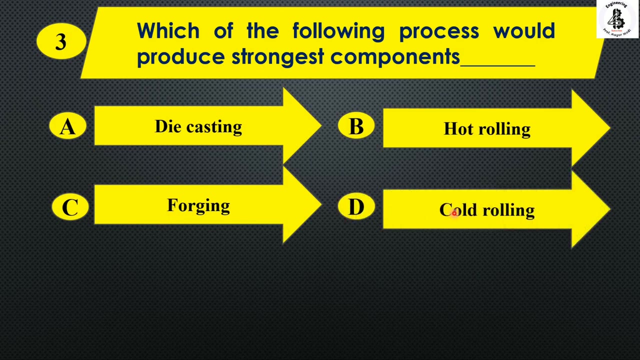 Next, which of the following process would produce strongest components? Option A- die casting, Option B- hot rolling, Option C- forging and option D- cold rolling. So basically, if you want to talk about strongest components, so forging process, that will be. 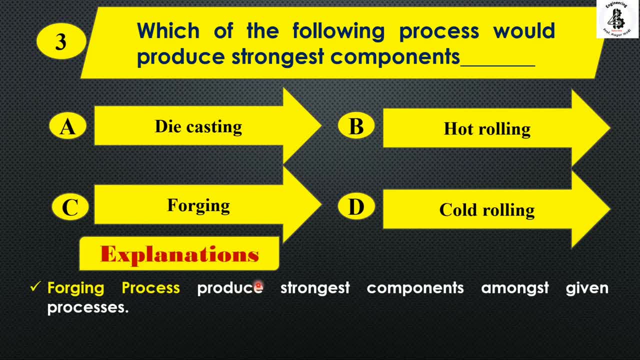 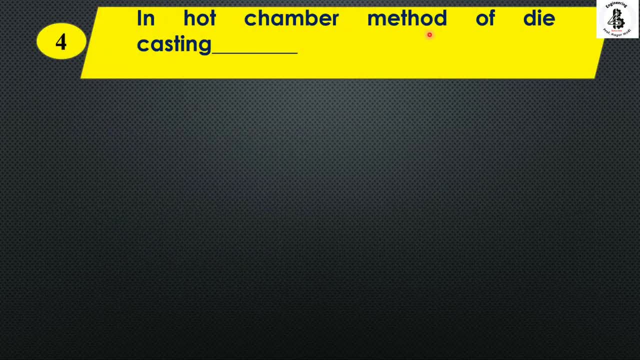 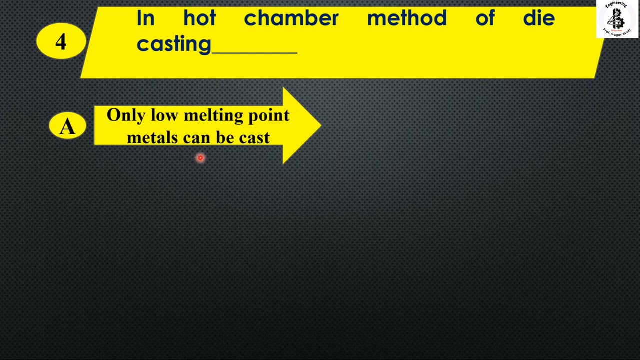 preferred for the various manufacturing processes. So the right answer is: option C: forging The next in hot chamber. method of die casting. option A: only low melting point metals can be cast. Option B: high melting point metals can be cast. 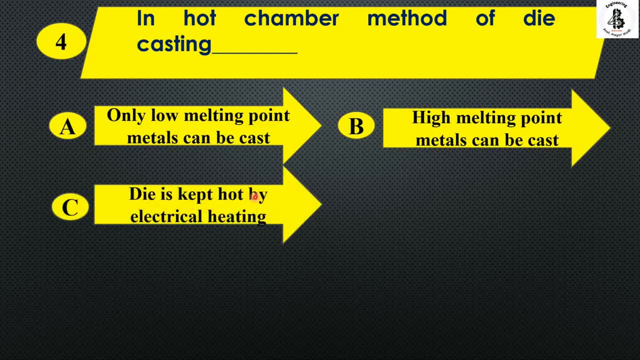 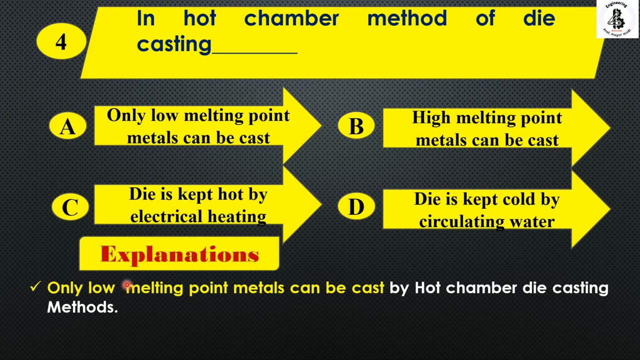 Option C- die is kept hot by electrical heating And option D- die is kept cold by circulating water Says from the name hot chamber die castings. So only that will be feasible with a special coffee reactor. So we know that the number of models or incidents is libraries. And in cases like the word room, coal mill, copper mill, ox, importante schedules, etc. for die casting the materials will be made of high capac Baker or coal gallic ore as per the power condition, store Standardidi裝 and cultivating process. 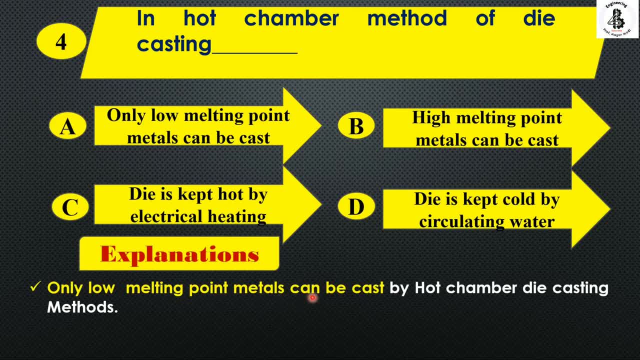 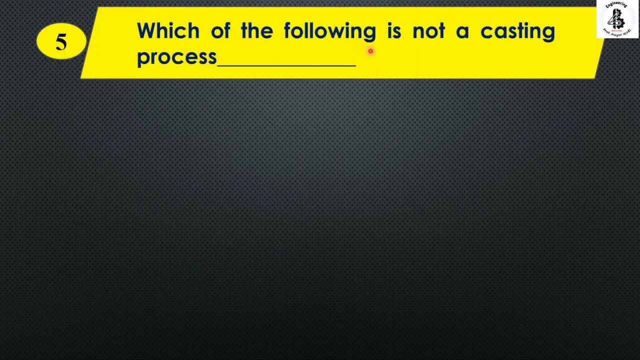 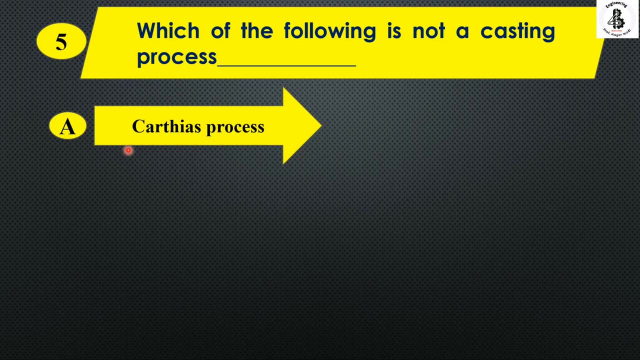 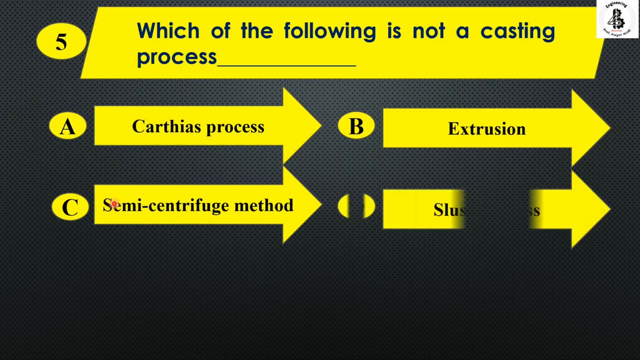 to a low melting point, matters can be cast. So the right answer is option A. Next, which of the following is not a casting process? Option A- partious process, extrusion process, option C- semi-centrifugal method and option D. 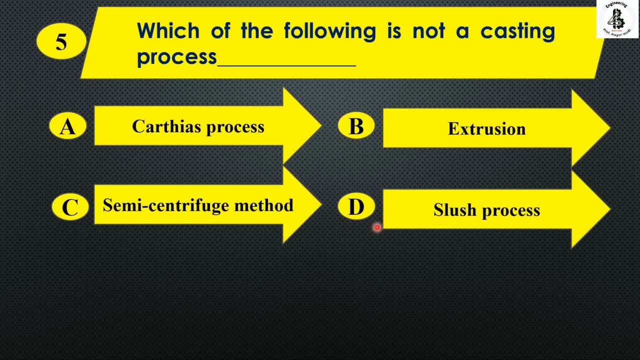 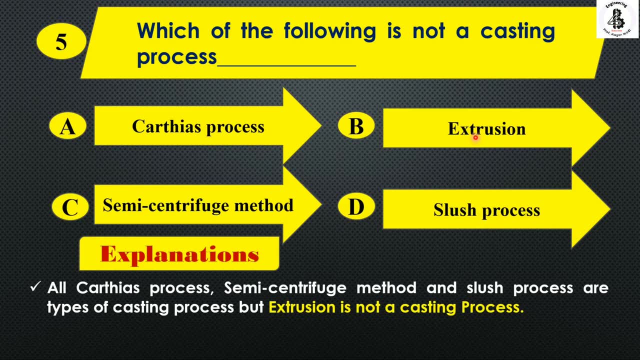 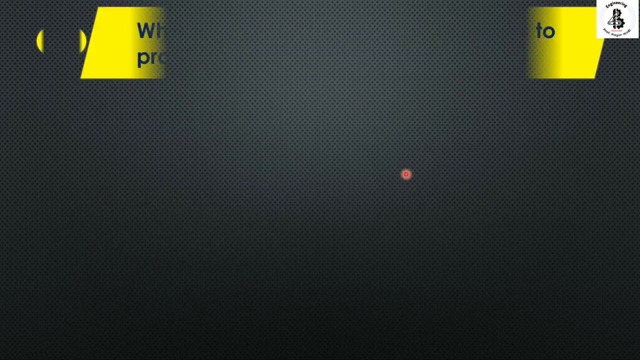 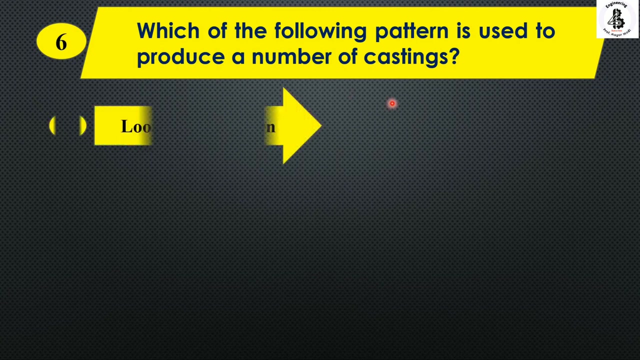 slush casting process. So basically, in that case, the extrusion that will be not considering as a casting process. So that will be considering as a forming process. So the right answer is option B. Which of the following pattern is used to produce a number of castings? Option A: 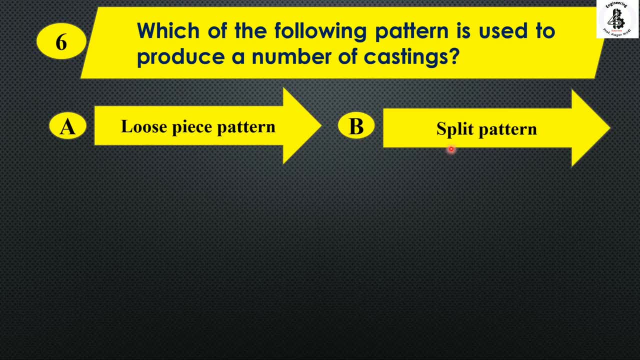 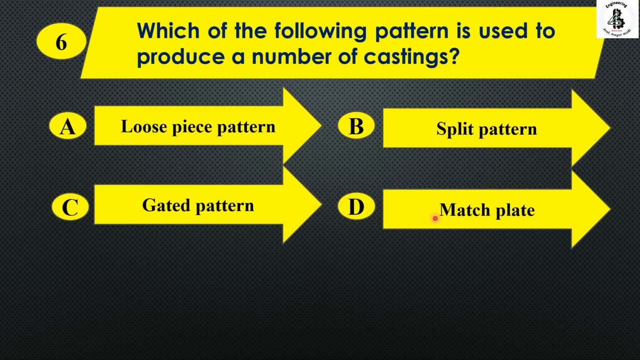 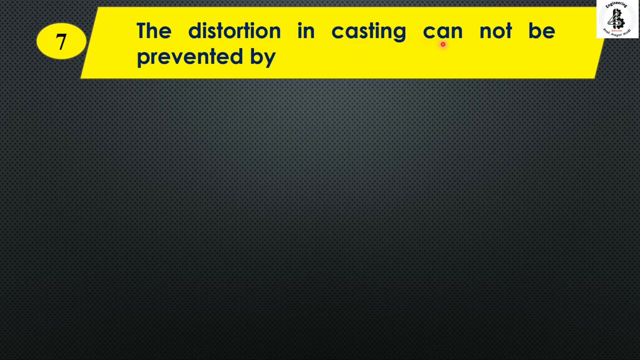 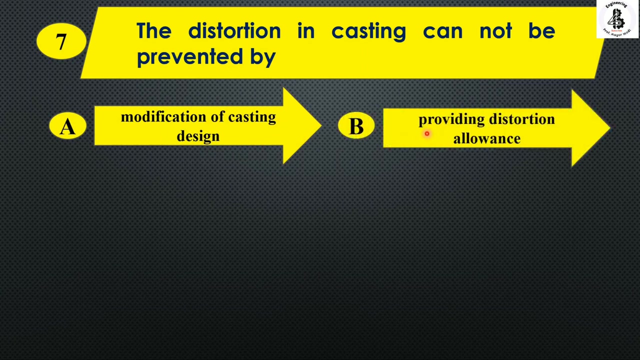 loose piece pattern, option B, split pattern, option C- gated pattern and option D, match pattern. So basically gated pattern that will be used to produce a number of castings. So option C. Then next, the distortion in casting cannot be prevented by option A- modification of casting design, option B- providing distortion. 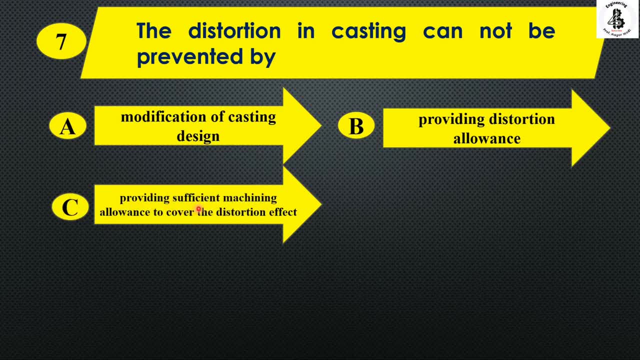 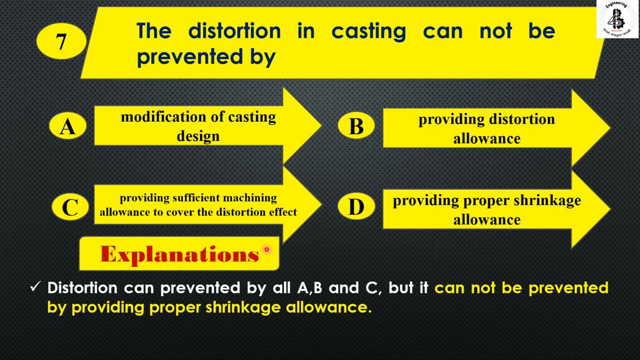 allowances: Option C providing sufficient machining allowance to cover the distortion effect and option D providing proper shrinkage allowances. So basically, in case of distortion can be prevented by all the A, B and C but cannot be prevented by providing proper shrinkage allowances. 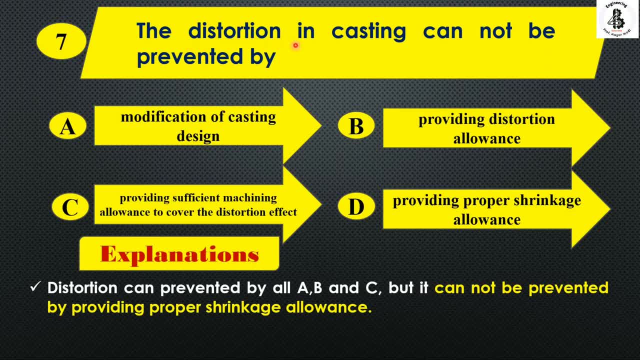 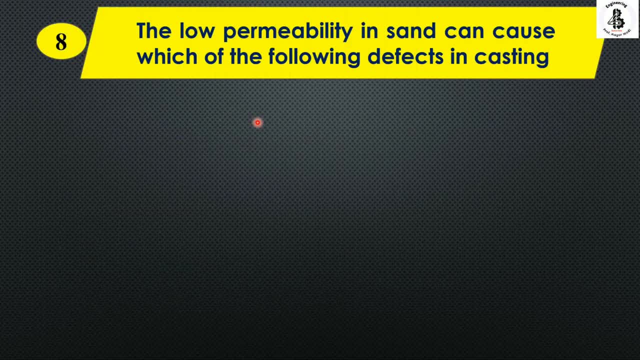 So here that will be. question is related with a. the distortion in castings cannot be prevented, be prevented, so the right answer is option d. the next: the low permeability in sand can cause which of the following defects into the casting: option a- rough surface. option b: blow holes. 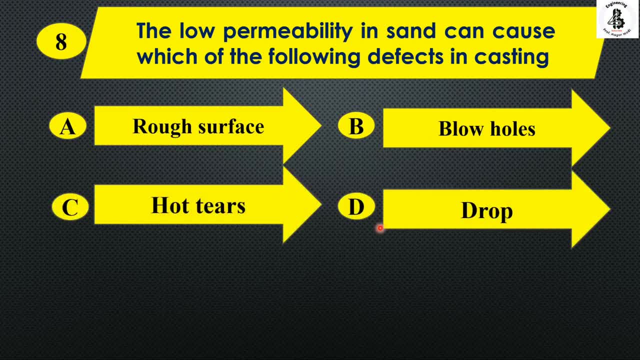 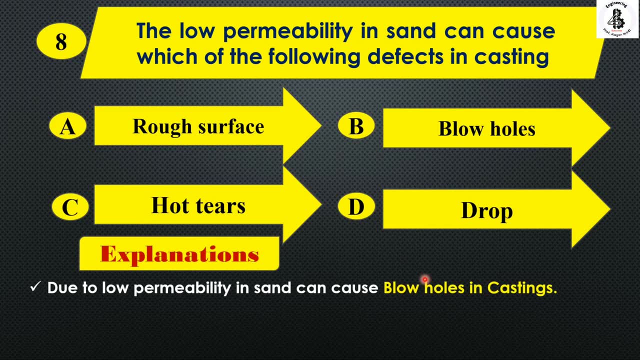 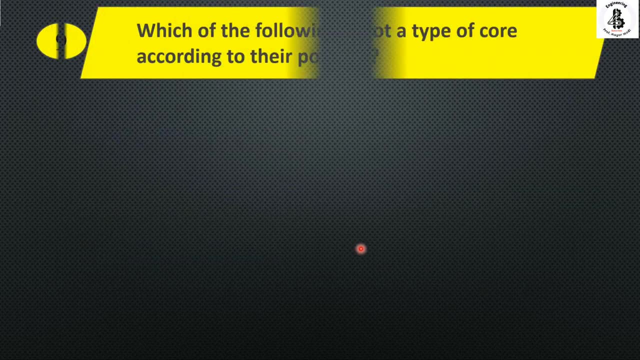 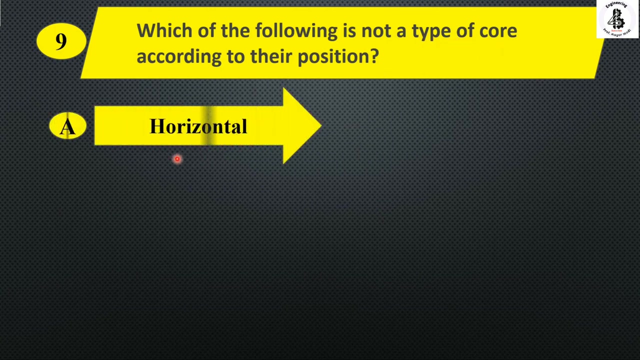 option c: hot tears and option d: drop. so basically, with respect to low permeability sands, that will causes a blow holes into the castings. so option b. then next question: which of the following is not a type of core, according to their position? option a- horizontal. option b- vertical. option c- inclined. 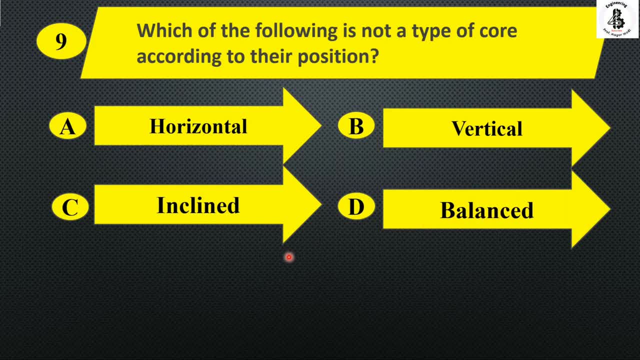 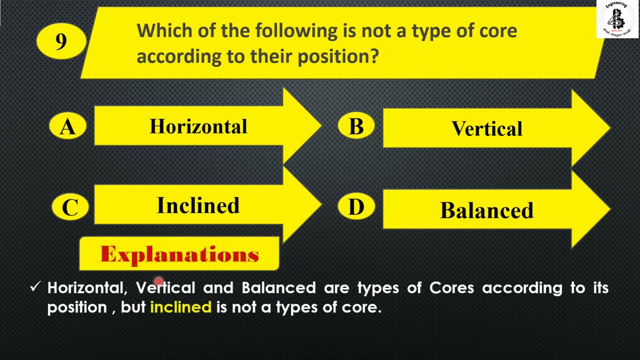 and option d balance says from the classifications of different kind of cores with respect to the positions, the horizontal, vertical balance, that all are the types of cores according to its positions, then more like a key score than hanging cores, but as per the given options, the incline that will be. 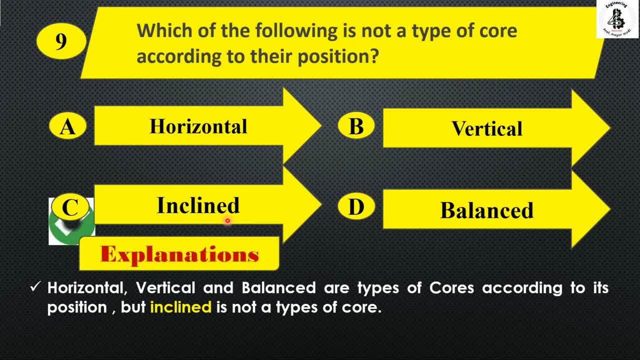 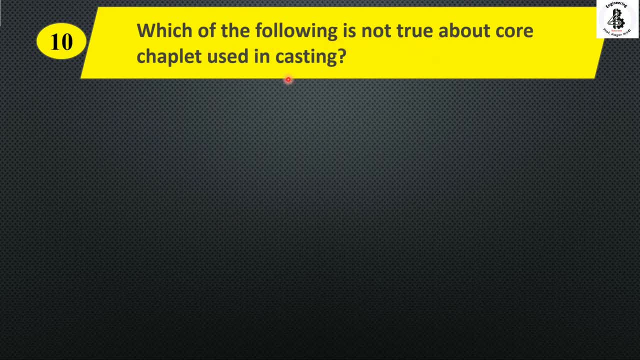 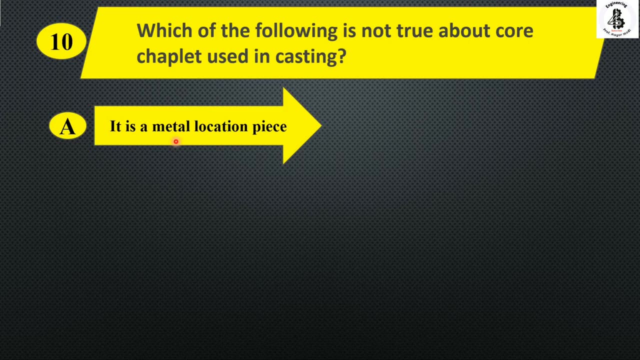 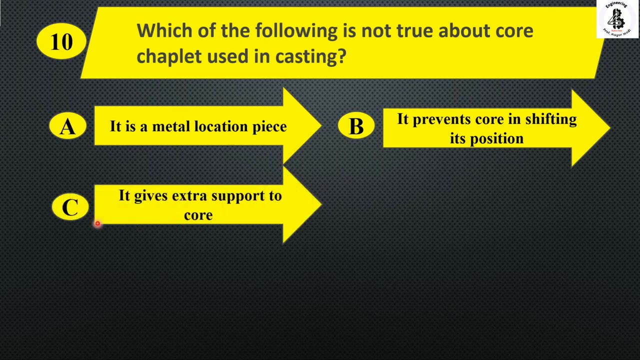 not a type of core. so option c, the next. which of the following is not true about core chaplet used in casting? option a: it is a metal location pieces. option b: it prevents core in shifting its position. option c: it gives extra support to core. and option d: it is removed after casting. 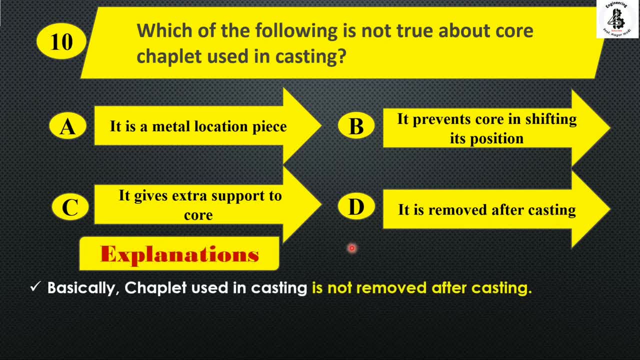 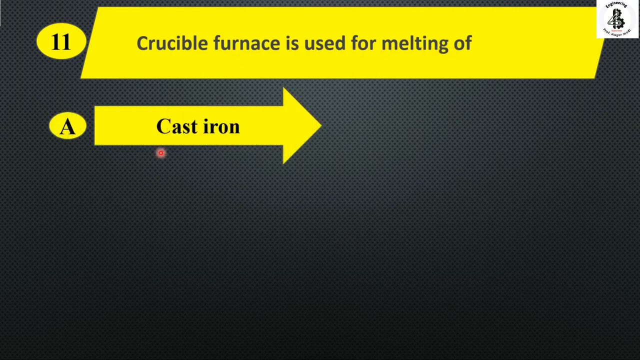 so basically, chaplets used in castings is not removed after the castings. so the right answer is that will be d: it is removed after the castings. that is not a true about a core chaplet used into the castings. next, crucible furnace is used for mediting of option a, cast iron. option b, copper. 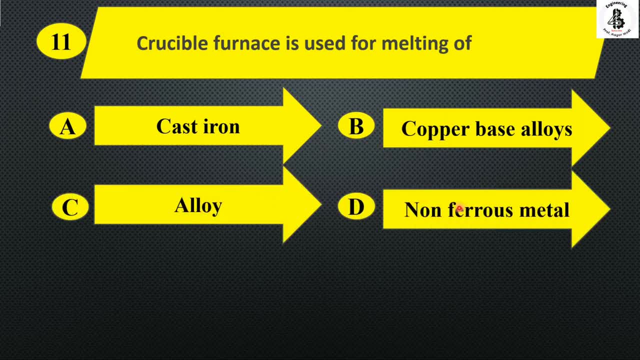 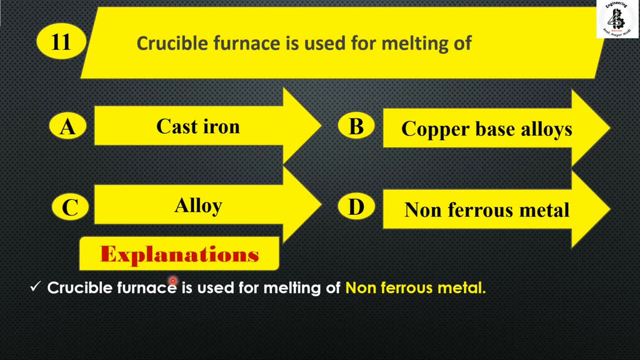 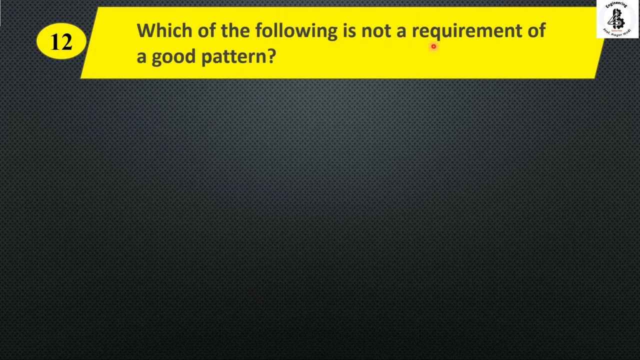 beige alloys, option c- alloy and option d- non-ferrous metal. so basically, the application of crucible furnace is used for mediting of non-ferrous matters. so right answer is option d, the next: which of the following is not a requirement of a good 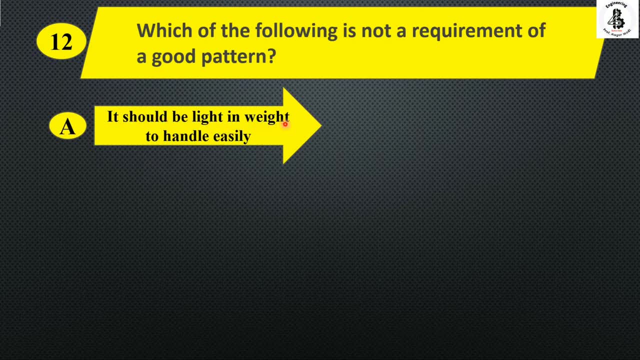 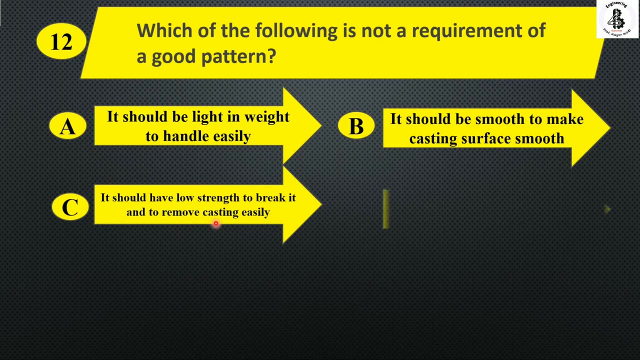 pattern. option a: it should be light in weight, to handle easily. option b: it should be smooth to make casting surface smooth. option c: it should have low strength to break it and remove casting easily. and option d: none of the above. so basically it should have low strength. 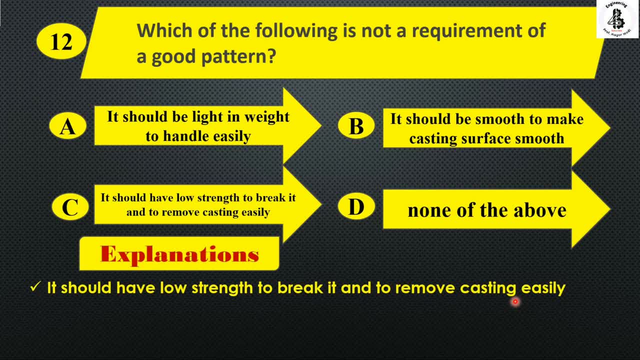 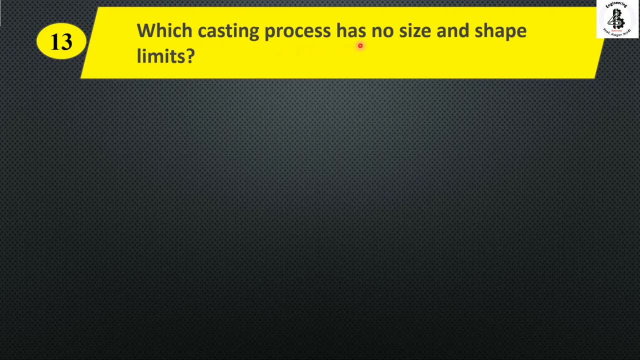 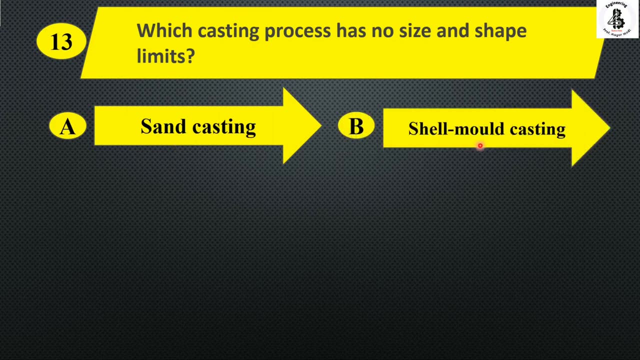 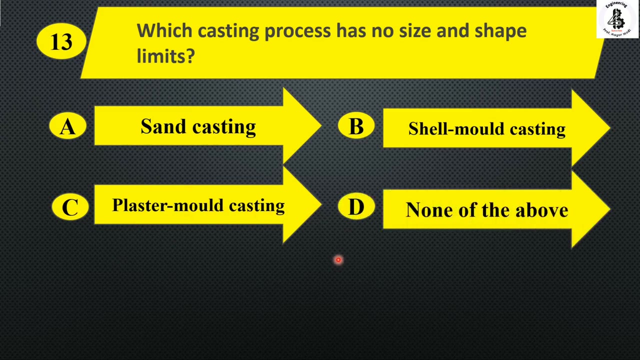 to break it and remove the castings easily. so that is the right answer. option c: the next, which casting process has no size and shape limits: option a- sand casting. option b- cell mold casting. option c- plaster mold casting and option d- none of the above. so basically, there will be the no limitation with respect to the 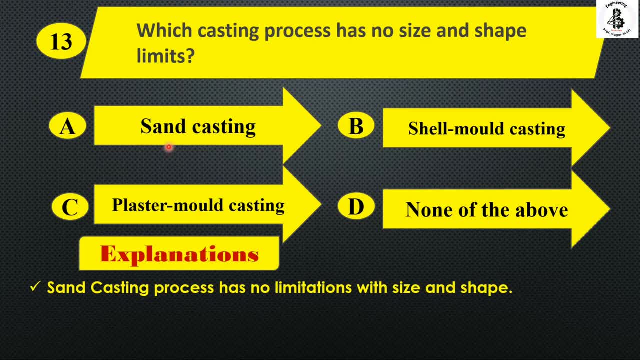 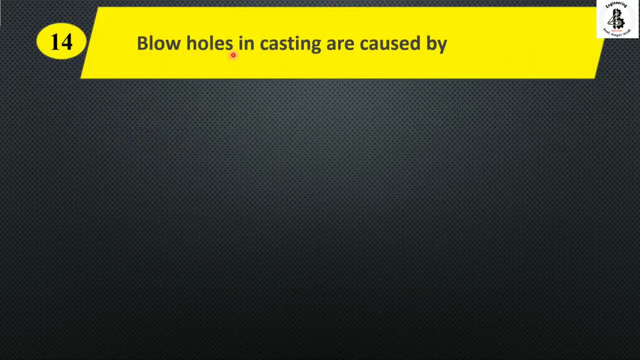 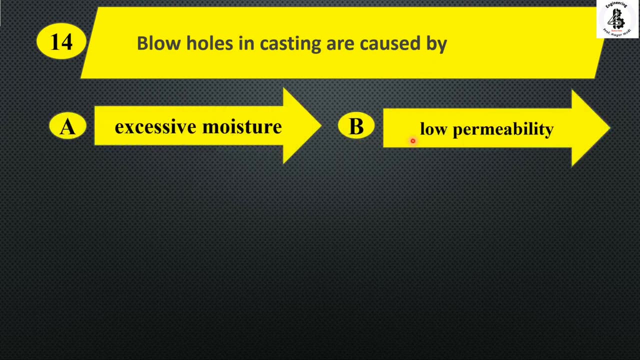 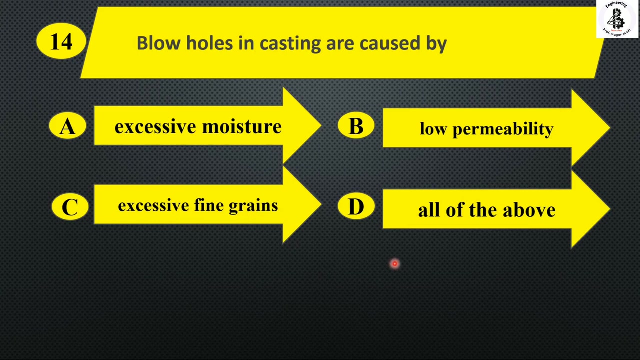 shape and size. so you should prefer sand casting process. so the right answer is option a, sand casting. the next question: blow holes in castings are caused by option a- excessive moisture. option b- low permeability, option c- excessive fine grains and option d- all of the above, so basically the blow holes that will be the one kind of defects into the 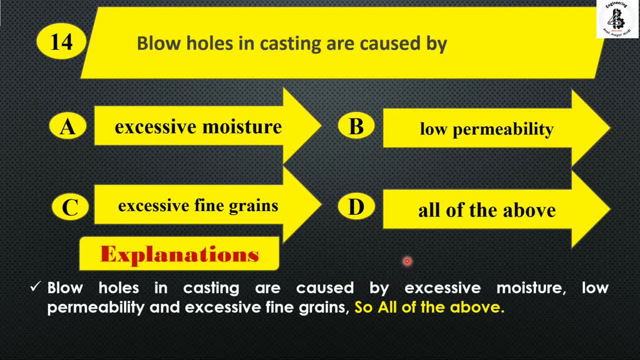 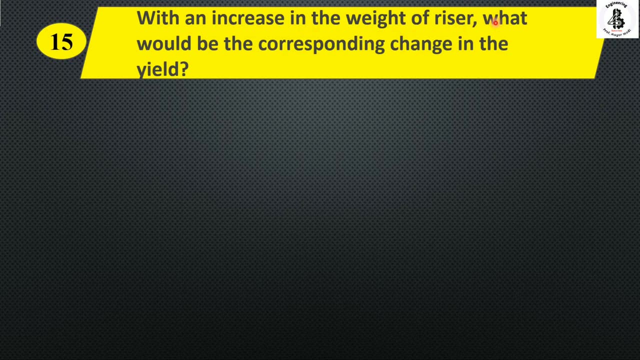 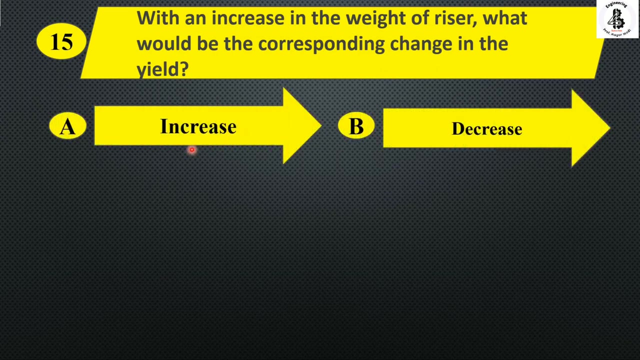 castings are caused by excessive moisture, low permeability as well as excessive fine grease. so the right answer is option d, all of the above. the next, with an increase in the weight of riser, what would be the corresponding change into the yield? option a- increase. option b- decrease. 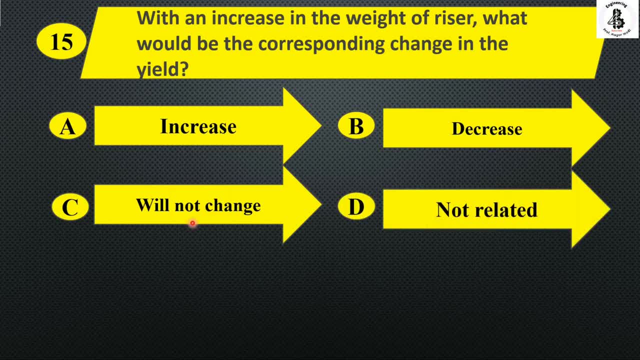 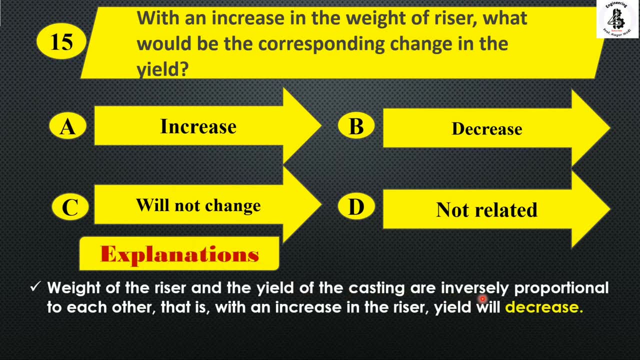 option c will not change and option d not related. so basically, weight of the riser and the yield of the castings are inversely proportional to each other. so that is the. with the increasing into the riser, the yield will, it will be decreases. so the right answer. 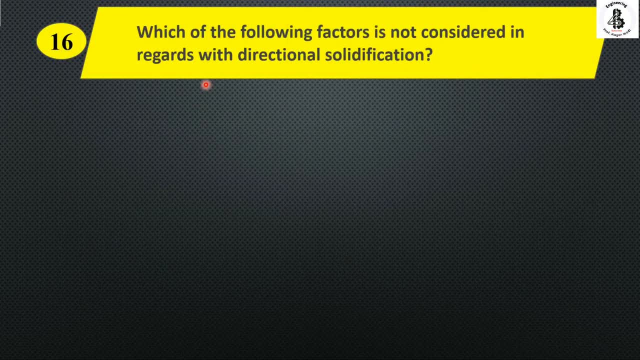 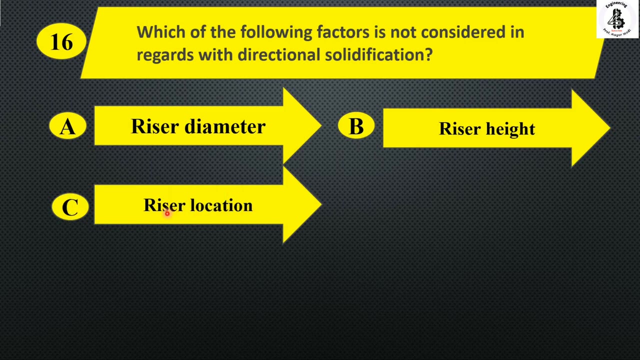 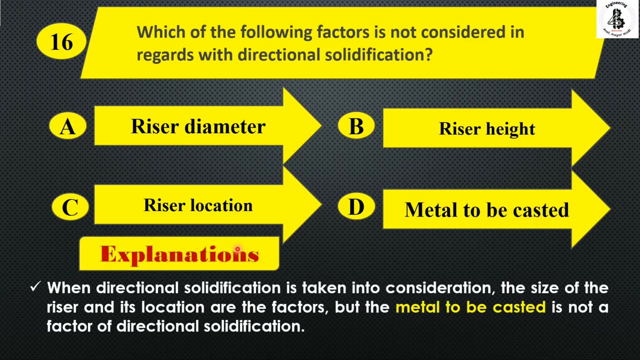 is: option b decreases. the next, which of the following factors is not considered in regards with directional solidifications? option a- riser diameter. option b- riser height. option c- riser location. and option d- metal to be casted. so, basically, when directional solidification is taken into the considerations the size of the riser as well as the location. 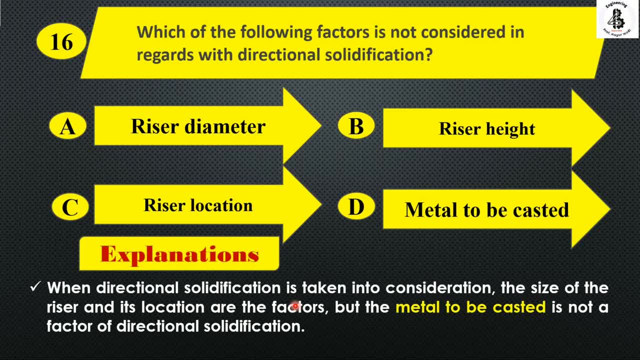 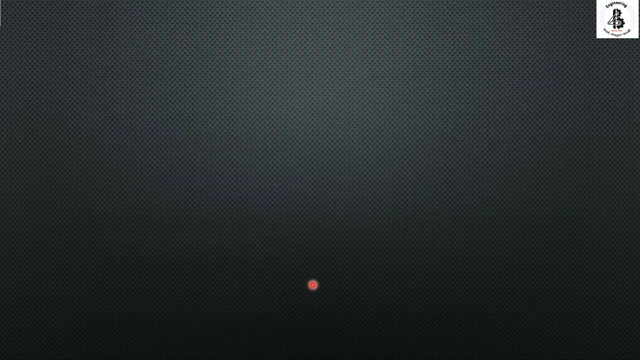 of the riser is taken into consideration. so the right answer is option d. the material to be casted is not a factor of the directional solidification process, so that will be not depends upon the which kind of compositions right. so the right answer is option d: matter to be casted, the next question. 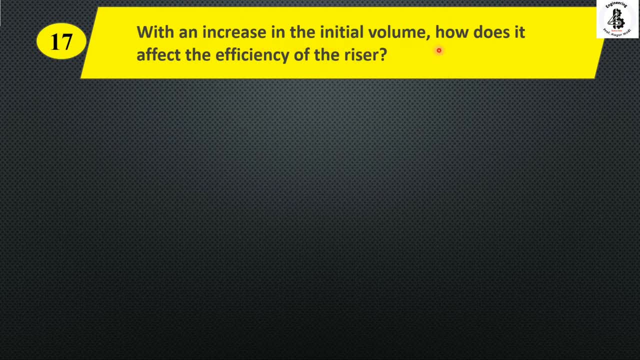 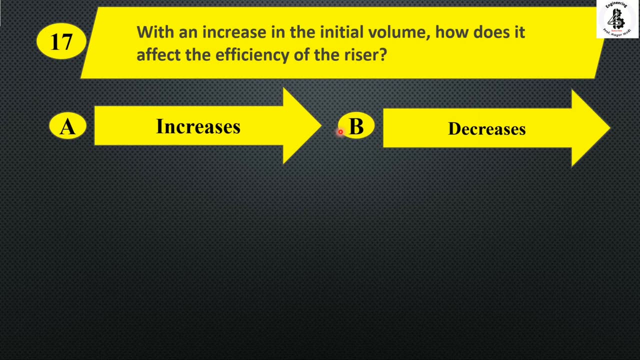 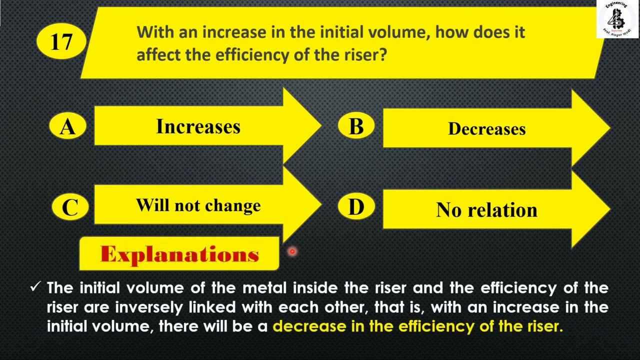 with an increase in the initial volume. how does it affect the efficiency of the riser? option a: increase. option b: decrease. option c will not change and option d not related. so basically, the initial volume of the metal inside the riser and the efficiency of the riser are inversely. 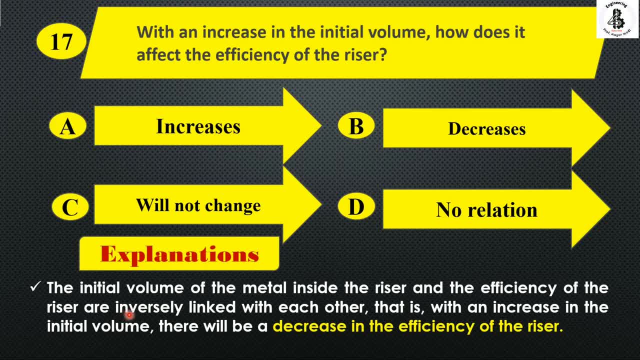 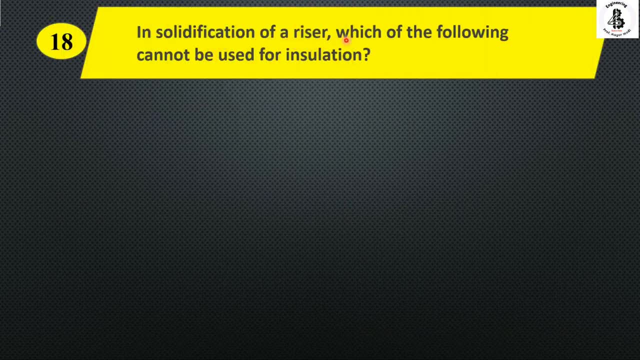 linked with each other so that with an increase into the initial volume there will be a decrease in the efficiency of the riser. so the right answer is option d decreases. so the right answer is option d- decreases. the next question: in solidification of riser, which of the following cannot be used for insulation? option a: insulation powder. 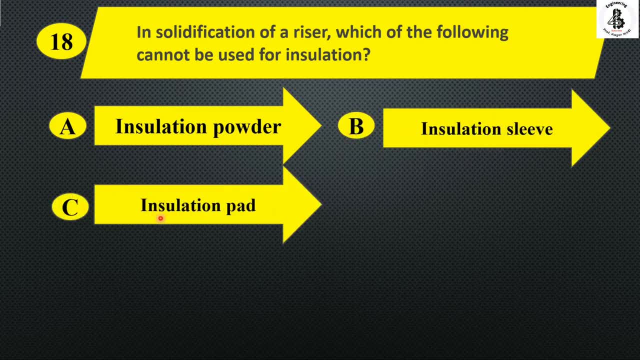 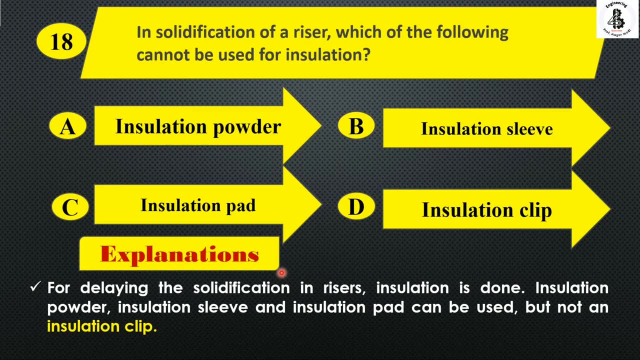 option b- insulation sleeve, option c- insulation pad and option d- insulation clip. so in case of the solidification of the riser, the insulation is done. so the insulation powder, insulation sleeves and insulation pad can be used, but insulation clips that will be not used. so right answer is: